Hello and welcome to MooMooMath. In this video I'd like to work on some proportion word problems And proportions are nice because you can take what is known and find what is unknown. Now, as I work these first couple examples, I'll go through a couple of helpful 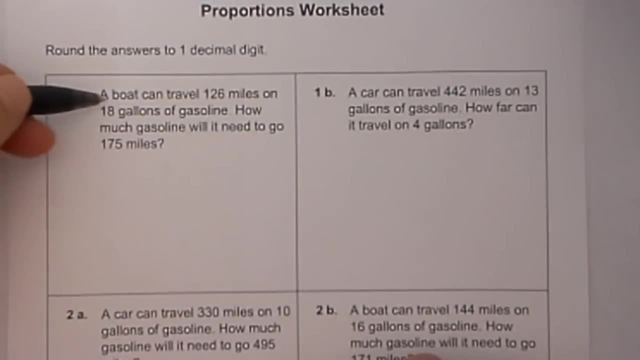 hints so you set these up properly. A boat can travel 126 miles on 18 gallons of gas. How much gas will it need to go 175 miles? So let's take what is known, and that is, if it travels 126 miles, that's going to take 18 gallons. Now one question is which. 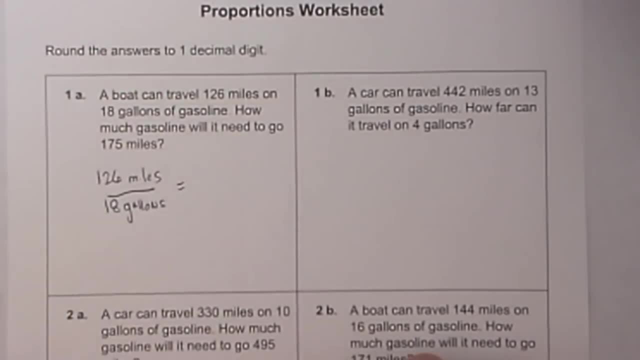 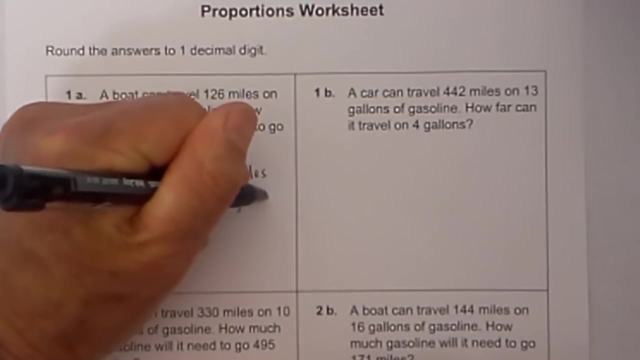 should you put on top the gallons or miles? But if you set the proportion up properly, it really will not make a difference. But what is very important, if you have miles on the top, here You must set what is equal to the same. So, if you'll notice, I have miles and miles. 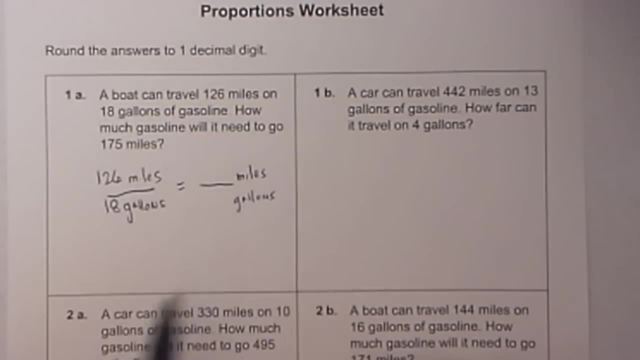 gallons and gallons. That's the most important thing. Now let's take what other information is given. I know that if I go 175 miles and I need to know how many gallons that will take, and I'm just going to set that as X, So I have it set up properly with the numbers. 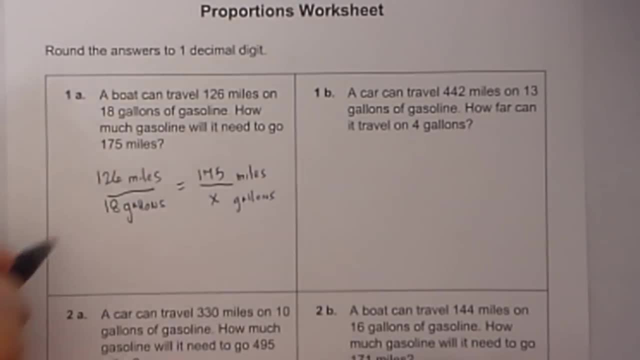 the same on the top and bottom. And then now I practice a cross box. So I take 175 times 18.. So I'll go 175 times 18, and then I'll go 126 times X. So I'll go. 126 times X is equal to, let's see, and 175 times 18. I've already done the math there. 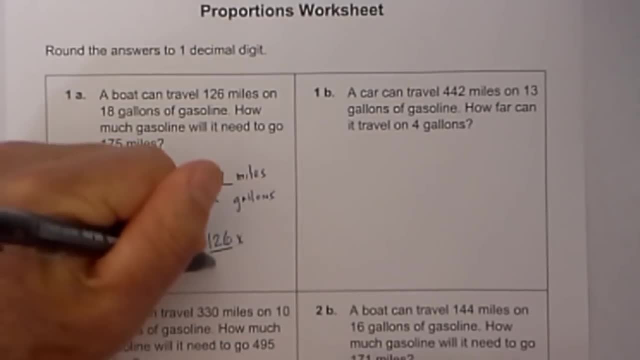 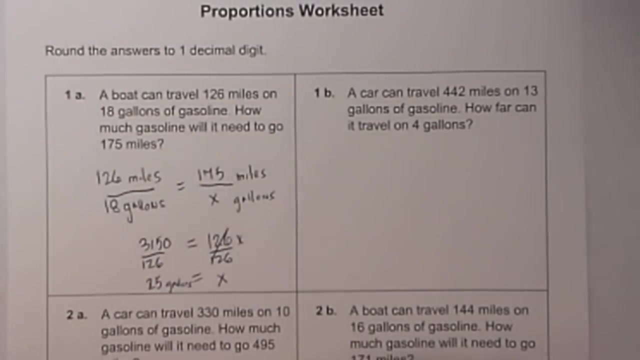 is 3,150.. I now isolate the X by dividing both sides by 126. And when you do that, the numbers cancel and X is equal to 25 gallons and that is going to be gallons. So it will take 25 gallons to go 175 miles. 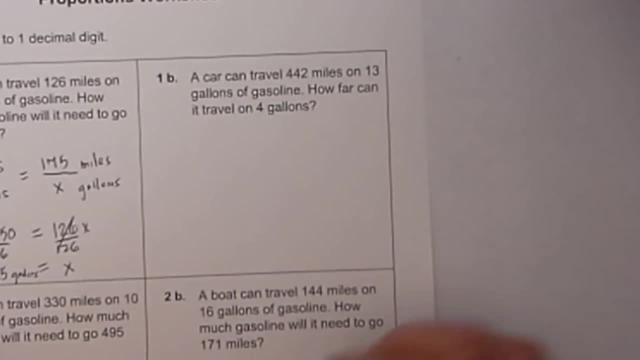 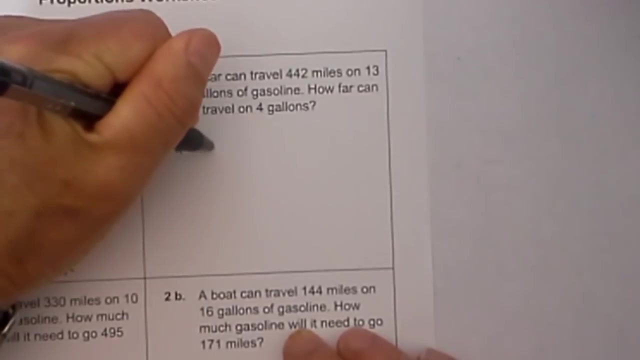 Let's look at another example which is very similar. This time a car travels 442 miles on 13 gallons. How far can it travel on 4.? So what I'm going to do is I'm going to go ahead and put miles on top again for 42 miles and, if you would like, you can set up the same. 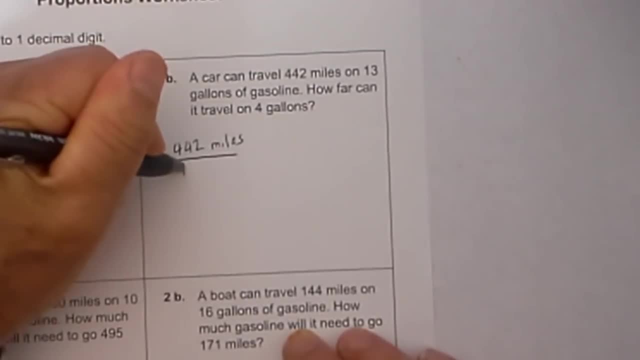 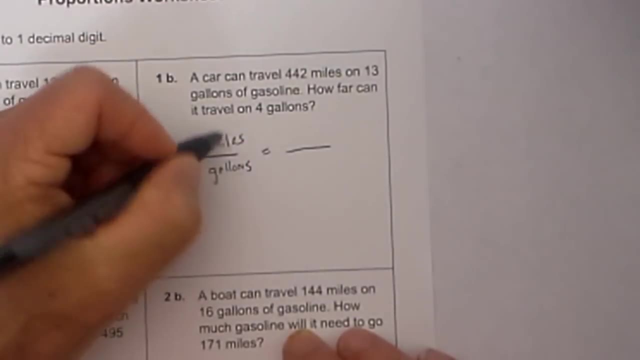 problem and put gallons on top and you will see, you will get the same answer. I am going to put gallons on the bottom. Remember, the most important thing is you set up the other fraction, the same, and I am going to put miles and gallons. 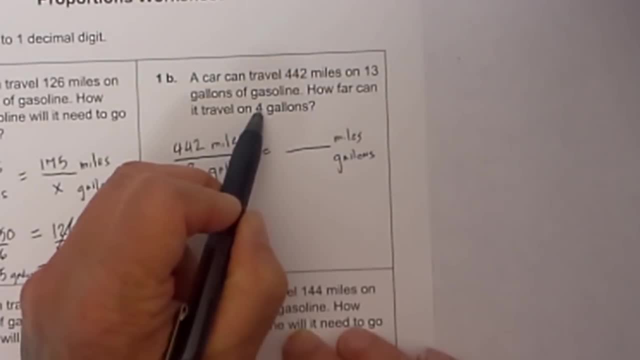 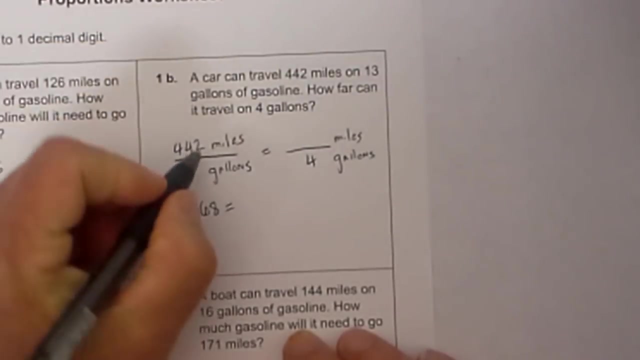 Now let's see what other information they have given us. How far can it go on? 4 gallons, So 4 is given. I then just complete a cross product and 442 times 4 is 1768 and then 13 times miles, excuse. 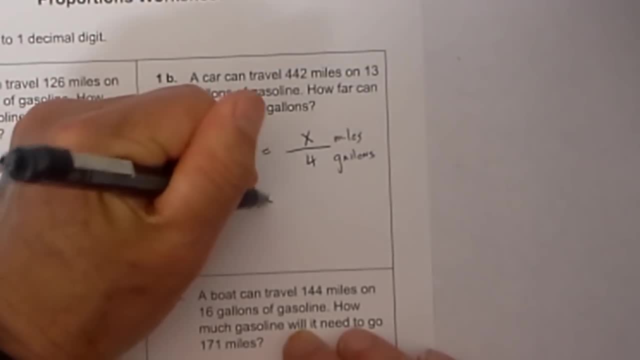 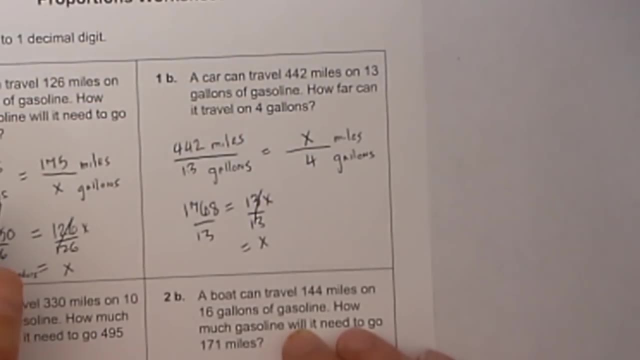 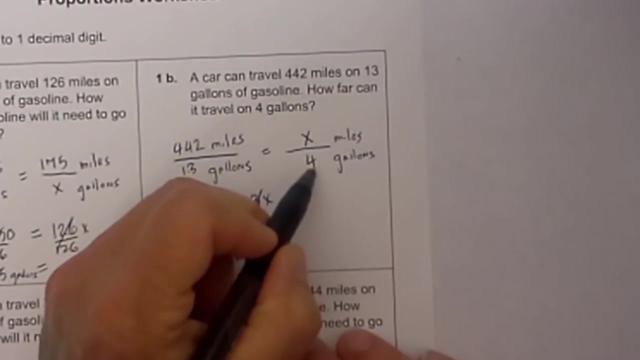 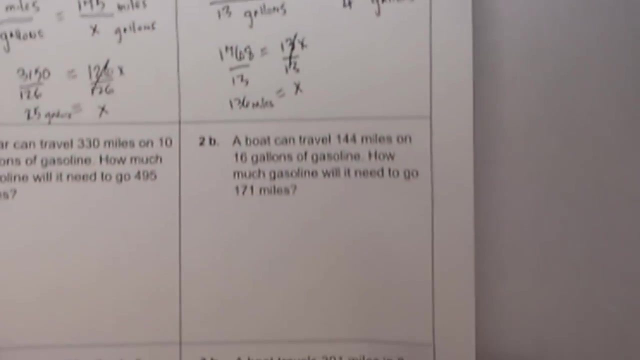 me. I left the x out. 13 times x is equal to 13x Divide each side by 13, and x is equal to 1768 divided by 136 miles. So it will travel on 4 gallons 136 miles. Let's go ahead and work two more of these, so hopefully you will get the hang of these. 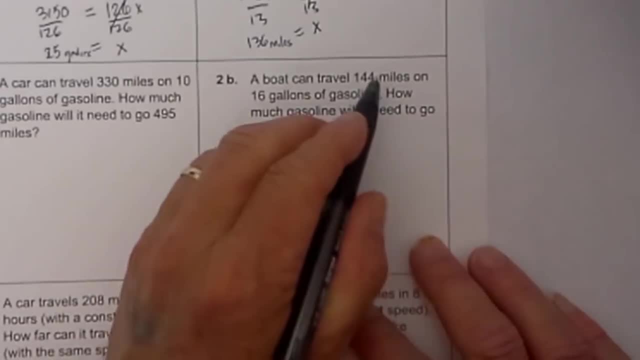 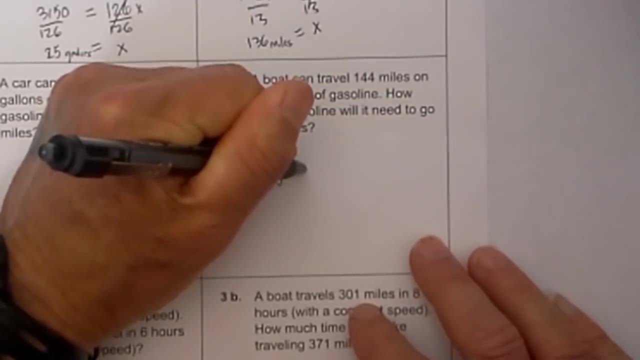 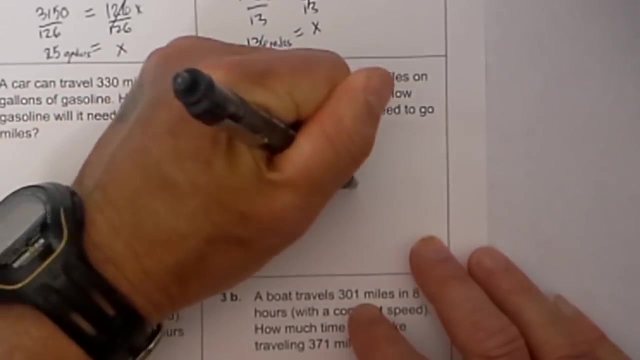 This next one is a boat can travel 144 miles on 16 gallons. This time I am going to put gallons on top. We know we have 16 gallons And with 16 gallons it can travel 144 miles. Okay, And I set the other fraction up: exactly the same gallons on top. 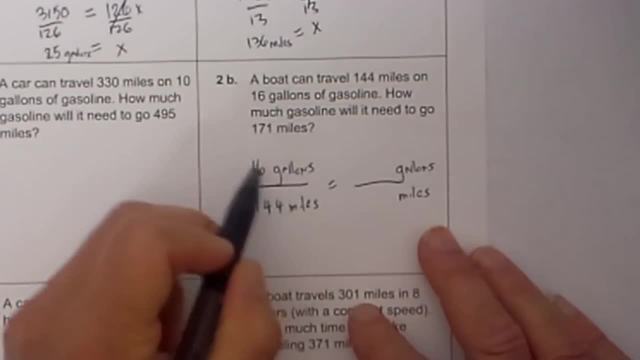 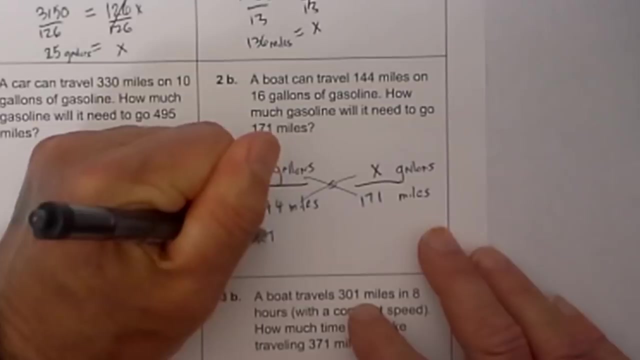 And let's do miles and what is given? it says it travels 171 miles and we need to know how many gallons that will take. We do a cross product: 171 times 16 is equal to 2736 is equal to 144x. 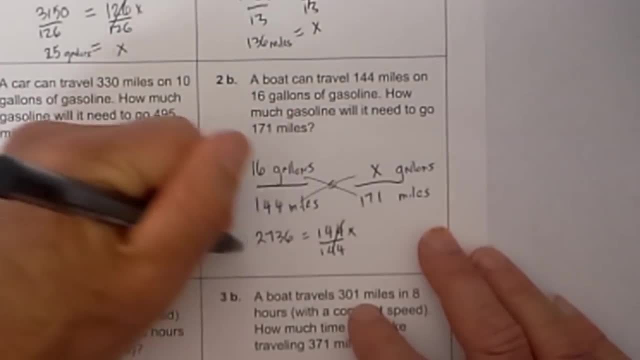 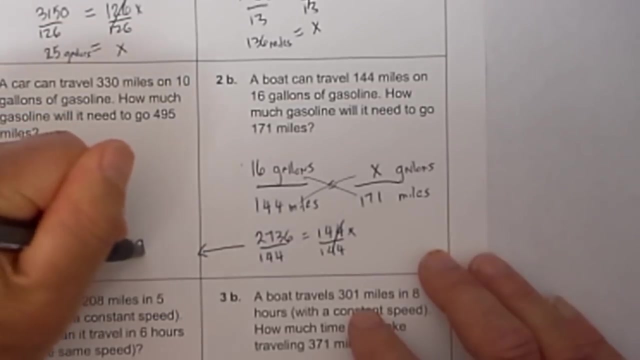 To isolate the x, we will divide both sides by 144.. These cancel in. 2736 divided by 144 is equal to: I am going to use this box right over here: x is equal to 19 gallons, So it will take 19 gallons to travel 171 miles.